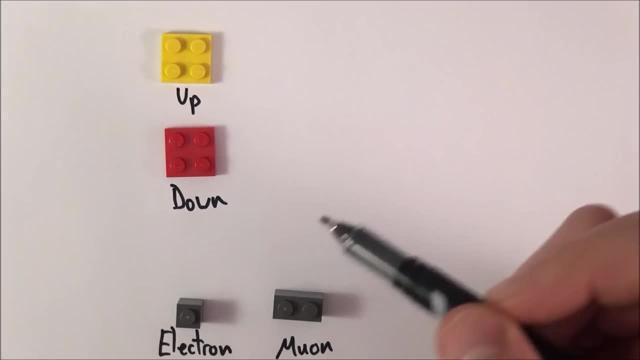 of hitting their surface. And along, as well as these electrons, we've had other things which were a bit like electrons, And we've had things which were a bit like electrons but they were neutrons, but they had no charge. And because they had no charge they were called neutrinos. 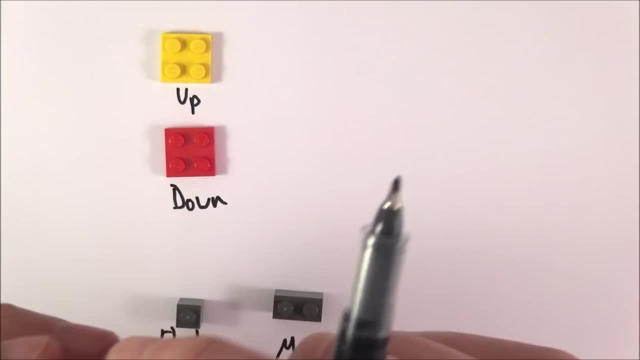 you know, neutron being neutral And effectively they're very small, So that's called a neutrino. So what I have here then, this little gray thing here, is my electron neutrino. So we have an electron neutrino, the electron a muon. Well, if we have an electron neutrino, 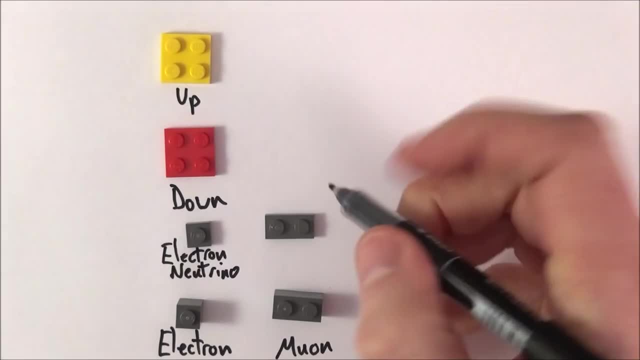 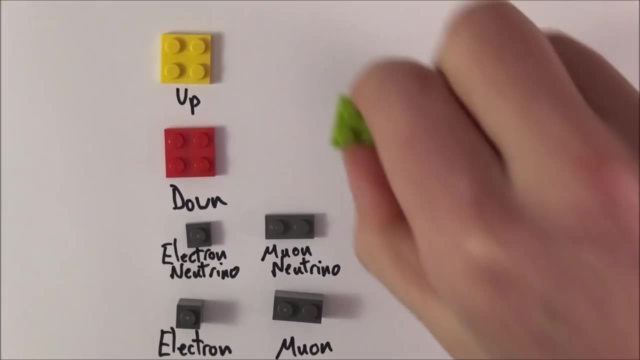 does that mean we also have a muon neutrino? Well, it does. yeah. And what they found is, as they discovered more and more particles. we had some particles which they called charm and some particles which had a very strange property, which we call strange quarks. 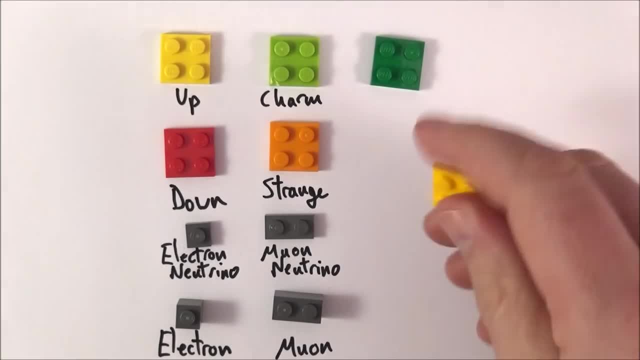 And as they looked more and more, what they found? they found some more quarks, okay, And here we have a quark at the top, which I'm going to call the top quark, and there's one just underneath it. 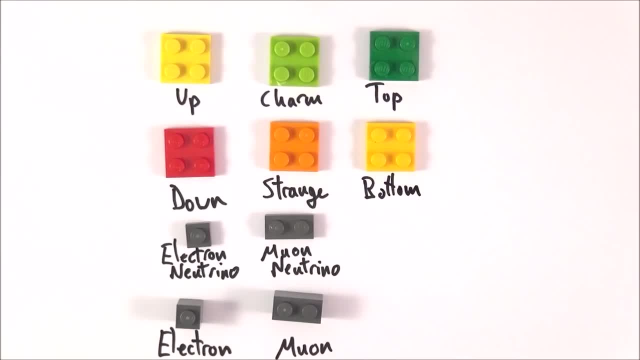 which I'm going to call the bottom, And you know these have other kind of properties And you know what we have now is we have kind of, you know, basically like a generation of matter here, another generation here, and that means there's also another particle. 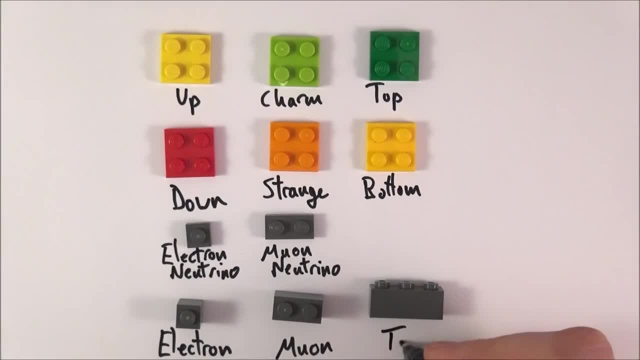 which is like an electron. Now this one here is called a tau particle. Now, a tau particle is a negative particle, but this has a mass equivalent to, like you know, the mass of a gold nucleus. So it's basically an incredibly, incredibly heavy electron. 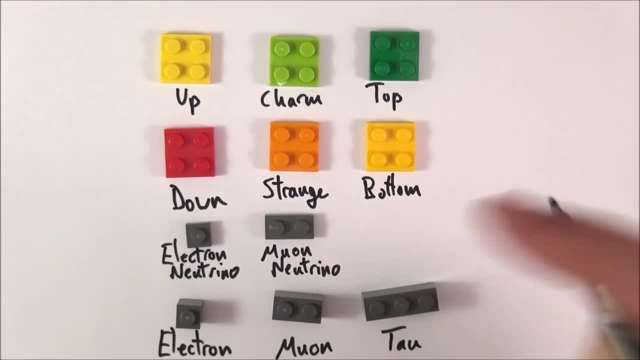 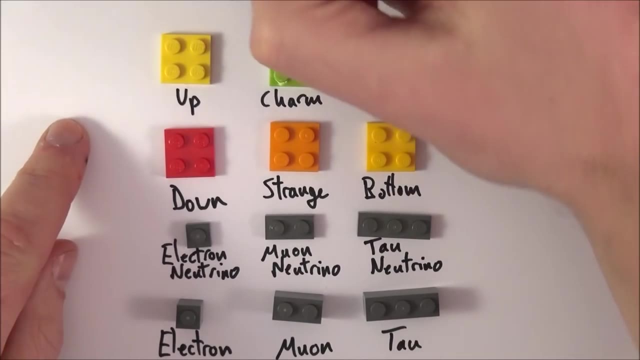 And that means not only do we have electron and muon neutrinos, we also have tau neutrinos. So what we have here are quarks at the top, and we also have a classification of particles that we call leptons, And what we find is that there's basically what we call three generations of matter. We've got the first generation. 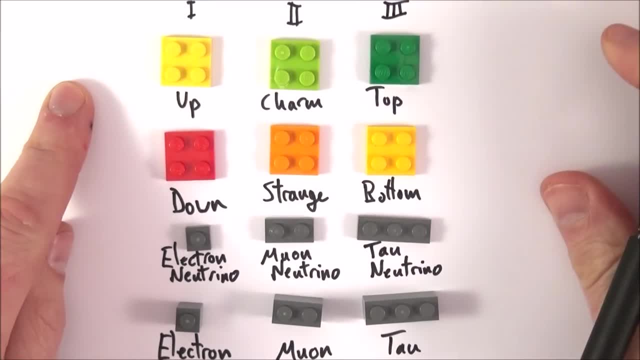 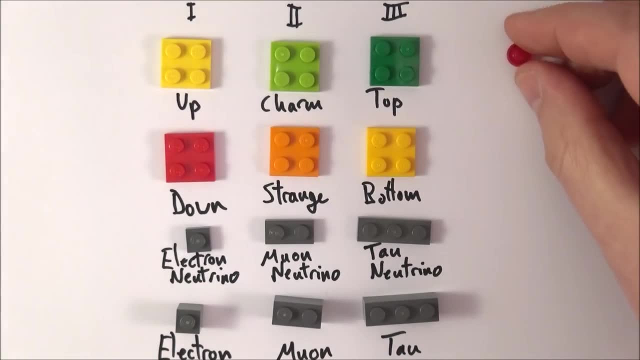 second generation and third generation. Why is that? I don't know, And I don't think anybody knows at the moment. There must be a reason for this, But what we also have on this model here is we have things that can carry the charge. 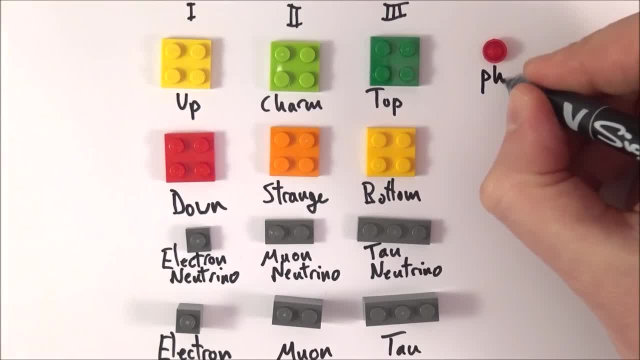 Now, first of all, this thing here is called the photon, and this is what you're very used to in terms of thinking about the eclipses, and this is what you're very used to in terms of thinking about the eclipses, about light, but a photon is what carries the electromagnetic force. Now there's also a particle. 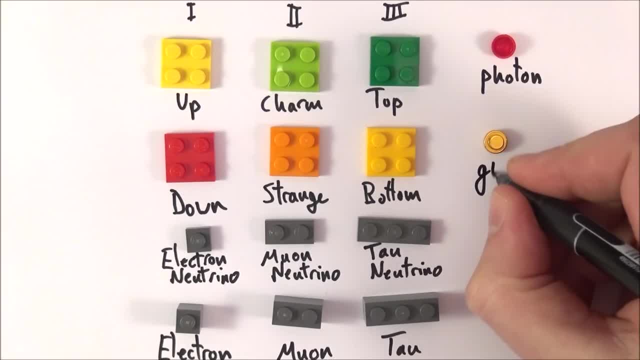 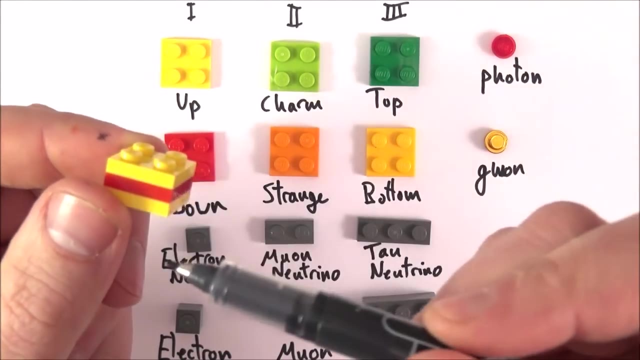 that carries the strong force and that's called a gluon because effectively it kind of glues the protons to the other protons inside the nucleus. But what we've now seen is that if inside a proton or a neutron we have maybe quarks inside, well actually these quarks also have a charge. 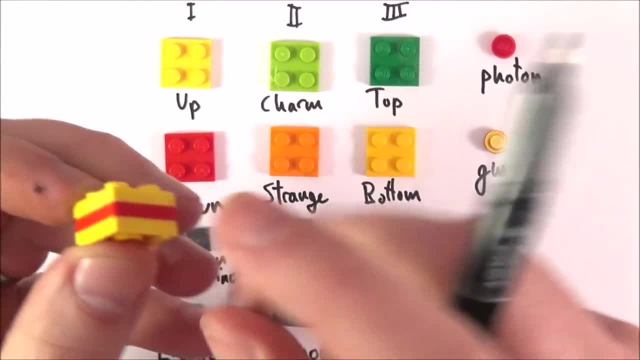 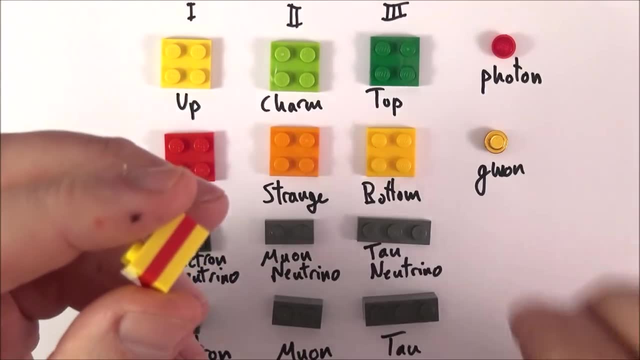 and in order to keep a positive quark near to another positive quark, there must be a force inside. Now, this force is only very, very short range, and this is what we call the weak force, And, again, the weak force is carried by a couple of bosons, and what we have here, then, are the W. 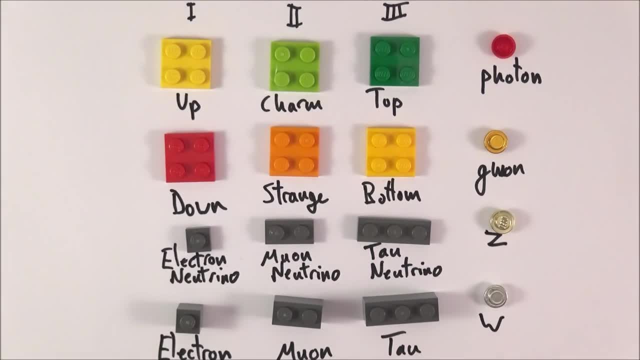 and the Z And this kind of seemed to make sense. What we have is basically a standard model of, but there's something missing. There's no reason, or we couldn't find a reason, why some of the things had mass, and that's where this thing here came along. This boson here is a boson that allows. 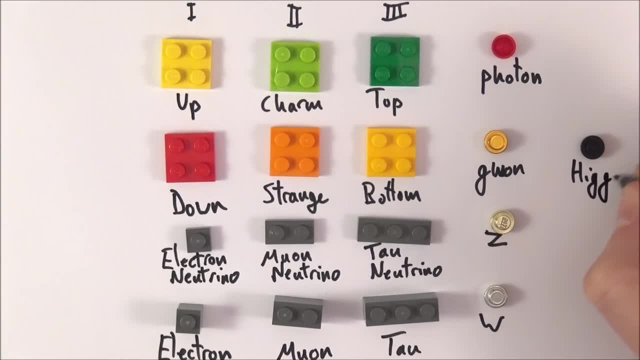 things to have mass and this is what we have now called Higgs, And you might have heard a lot of information in the press about the Higgs boson in the search book recently at CERN And really these things here are what we call bosons. 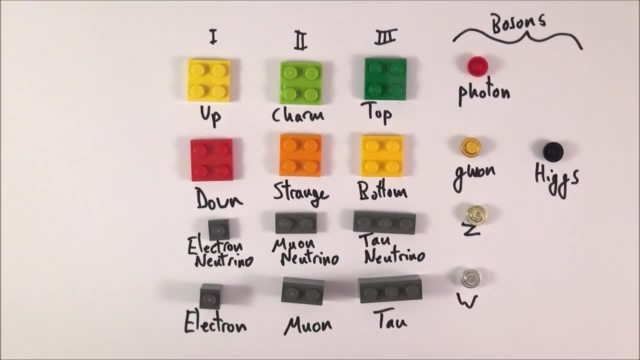 And it's this thing here which is called the standard model of physics. okay, Now, it's not just that we have protons, neutrons and electrons. What we find is that pretty much everything that we can see in the universe is made out of up quarks, down quarks and electrons. You know. 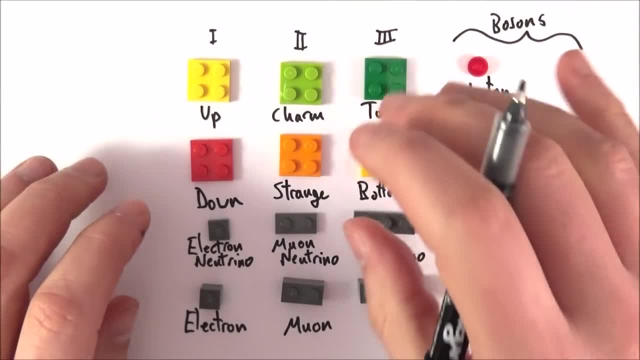 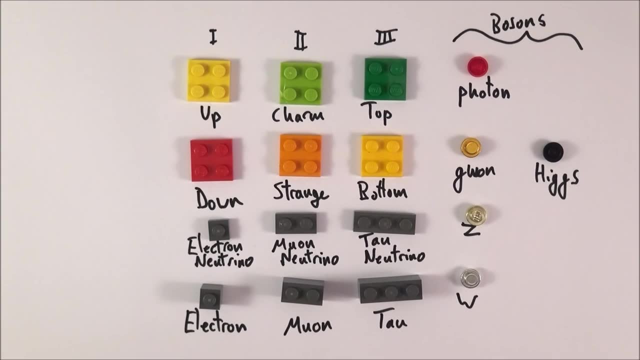 that makes up all the atoms, that makes up all of you. But these things here, they can exist, even if it's only for a short amount of time. they might come to being and then disappear back into energy, But this is a really, really fascinating part of physics, But this isn't. 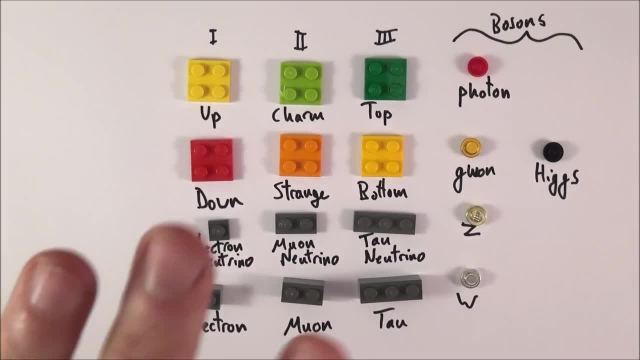 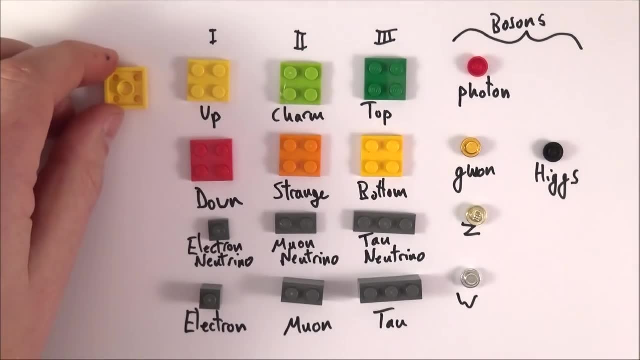 the whole model. Not only do we have up quarks and down quarks. in addition to all of this matter here we also have stuff called antimatter. Now, antimatter is- I'm just going to put them upside down- is a bit like normal matter, but it has an opposite charge and many other properties are. 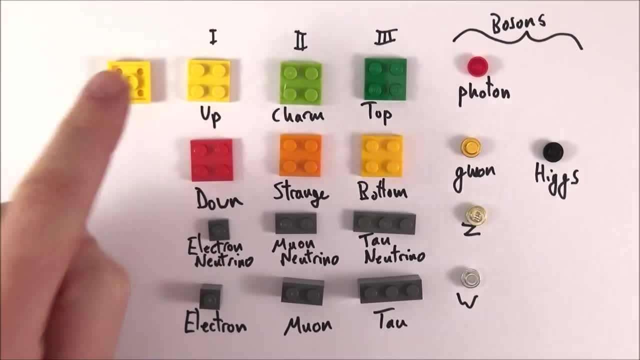 reversed. So, although we might have an up quark, we also have what we call an anti-up, And if we have a down quark, we have an anti-down. If we have an electron, we also have something that we call an anti-electron, In this case, 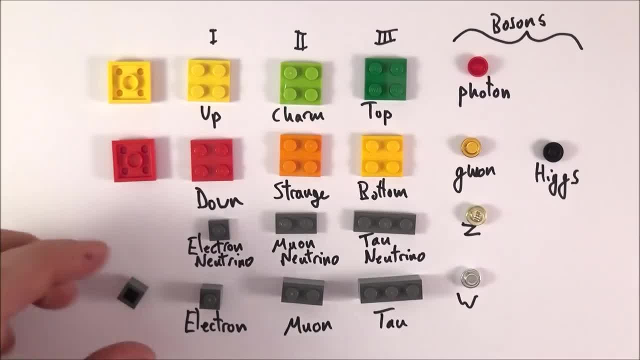 it might be called a positron, so a positive electron. So what we find is that, in addition to this, we have a mirror image of antimatter and the sort of antimatter equivalents, And basically, you know, they do exist And this is how we have things like PET scanners. so positron emission. 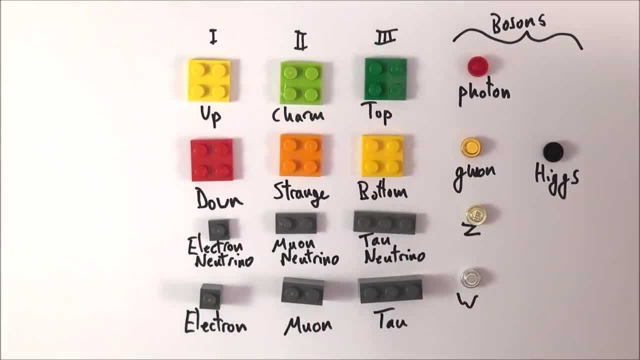 tomography, because these particles, these antimatter things do exist. Now again, if we classify things, we can classify things in two ways. First of all, the things at the bottom, in the middle of the graph are what we call leptons. Okay, and just like in biology, we classify things. 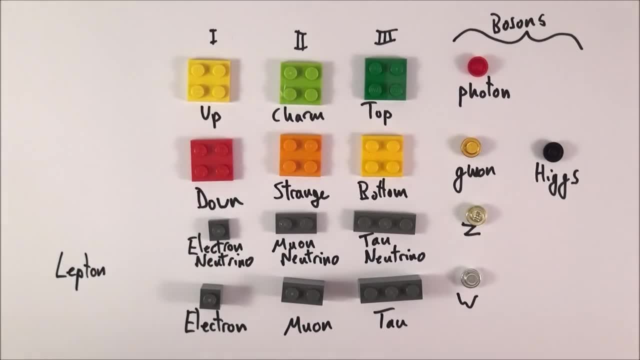 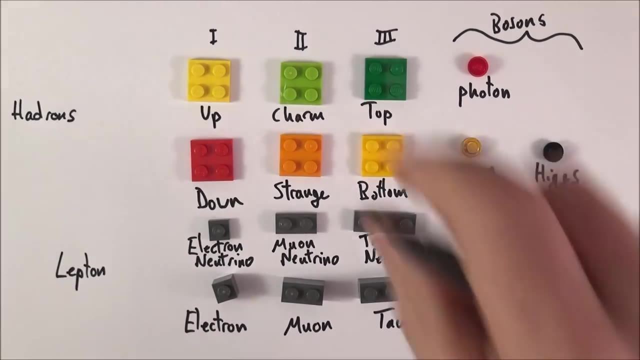 like birds and fish and so on. we can classify particles in different ways. Now at the top, using these six particles here, what we then do is we make up things called hadrons. Now there are basically two sorts of hadrons. Some hadrons are made out of three quarks, So 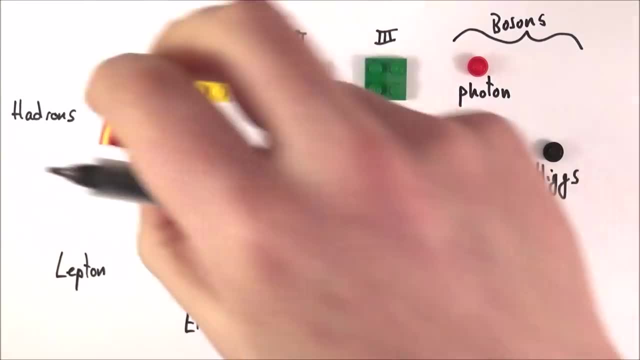 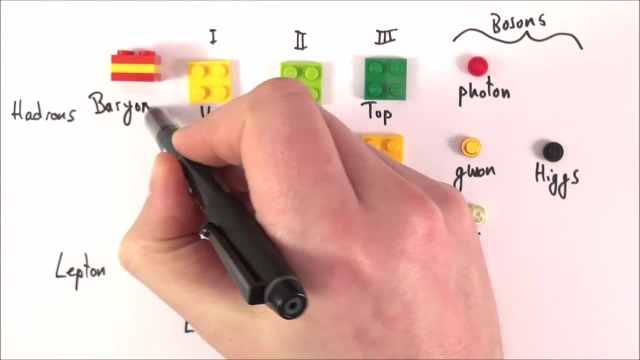 for example, if you have a neutron, it's made out of three quarks, and this is what we call a baryon. So a baryon is made out of three quarks, but we can also have things made out of two quarks. 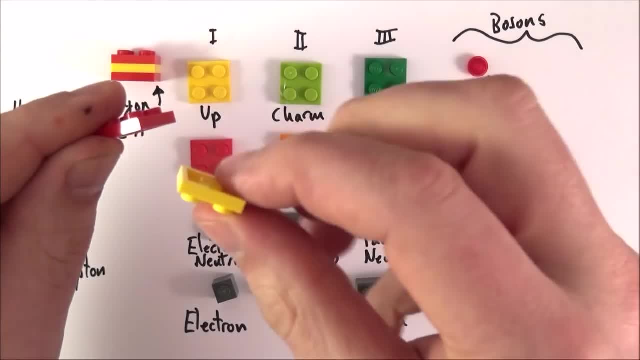 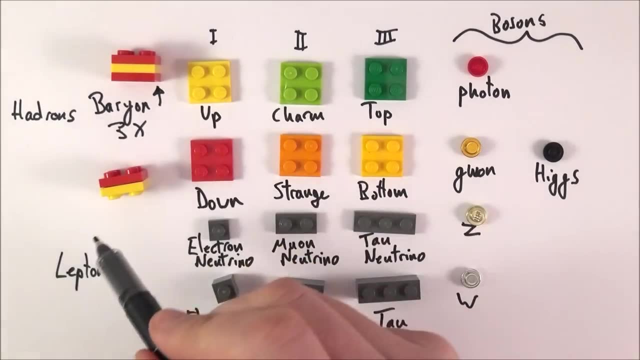 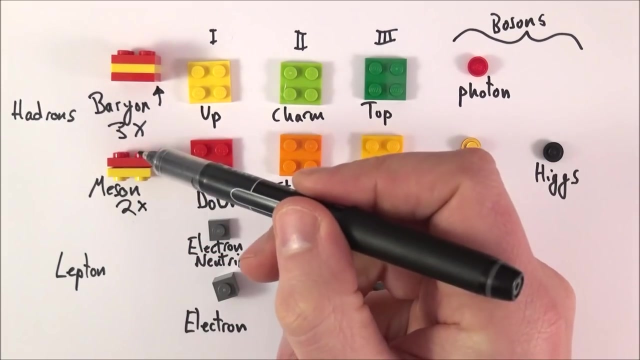 and in this case you might have a quark and an anti-quark, and basically, if you combine a quark and an anti-quark together, what we get then is something called a meson, And this meson is made out of two quarks: one which is a normal quark and another anti-quark. 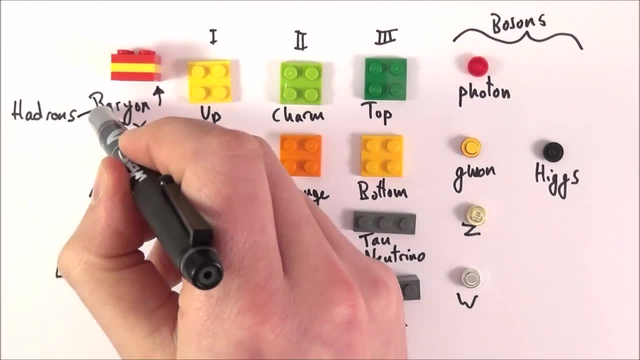 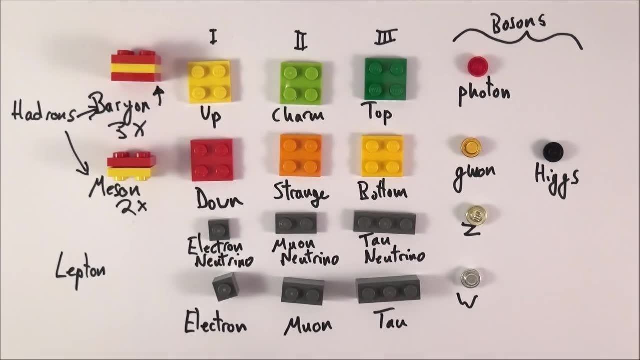 So, basically, what you can think about leptons, we can think about hadrons and hadrons there's two sorts: there's baryons and there's mesons. Does that make sense? Hopefully some of it does, but I guess this is probably going to give you many, many more questions, and this is a really really 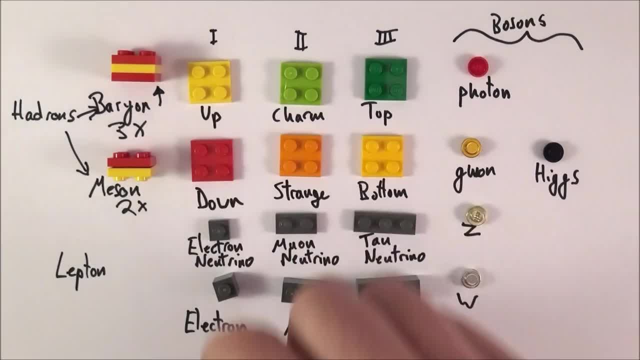 fascinating of physics at the moment. you know, people don't know all the answers. Why do you have three generations of matter? I don't know. How do you know how many generations of matter? electrons can turn into muons and so on? Okay, it does get complicated. but you know, this is a really really fascinating area.